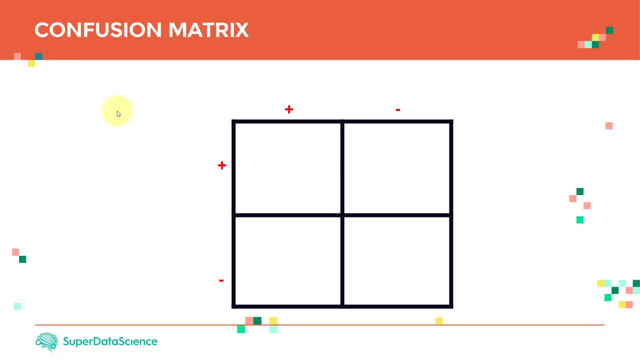 However, for classification tasks- which is, you know what we're going to apply here in this case study, because we're going to use logistic regression, which is mainly used for classification purposes- we're going to rely on what we call a confusion matrix, which is a matrix used to perform, basically to assess the performance of a classifier. 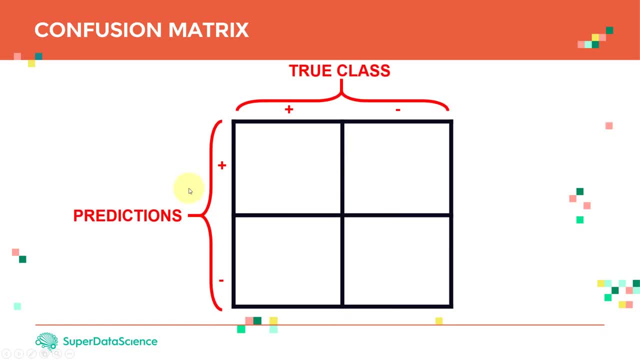 What we do here is we have simply our model predictions and we have what we call the true class. The true class are either positive or negative, one of two classes. The true class is either positive or negative. Simply put, that's what the model is predicting. That's what the model is telling me, okay. 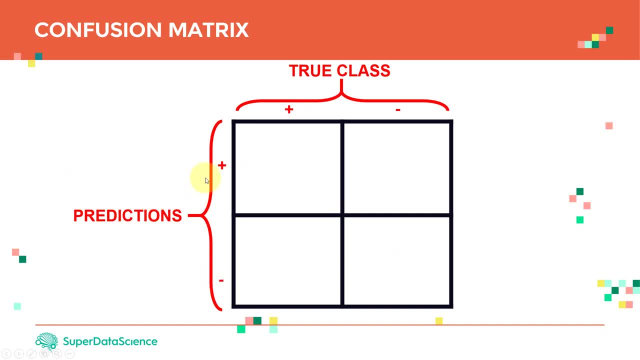 Like, for example, a patient is, let's say, has cancer, for example, or not. So if the patient has cancer, we're going to be here, If the patient does not have cancer, we're going to be negative. okay. 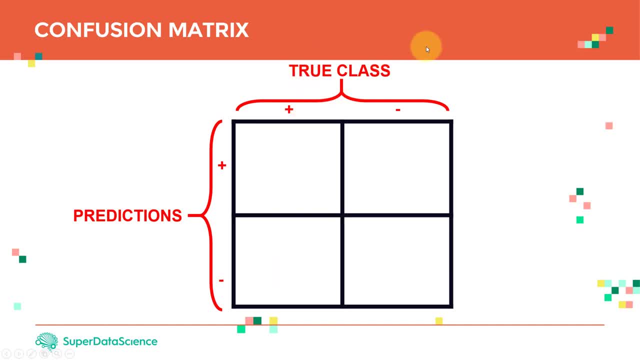 And here we're going to put the true class, which is either positive or negative as well. What happens is, if my model predictions match, if my model matches the true class, that's good. That's what we call it: true positives. 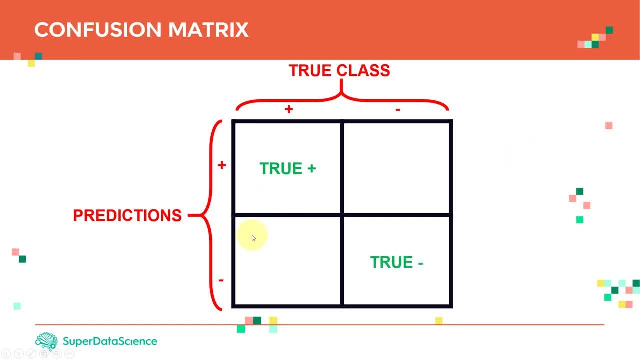 Then everything is great and you know, the model is perfect. And if, for example, the model says that the patient has doesn't have cancer- and the patient in fact did not have cancer as well, then we're going to call it true negative. So we're going to put the total number of correctly classified samples in here. okay, 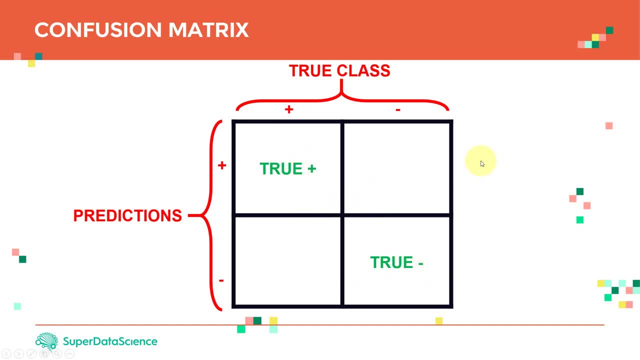 And now everything looks good. True positives and true negatives are perfect. However, you know models have problems- Models in general. sometimes they mess up. So let's take a look at some of the mess ups. Let's assume that the model predicted that the patient had cancer. okay, 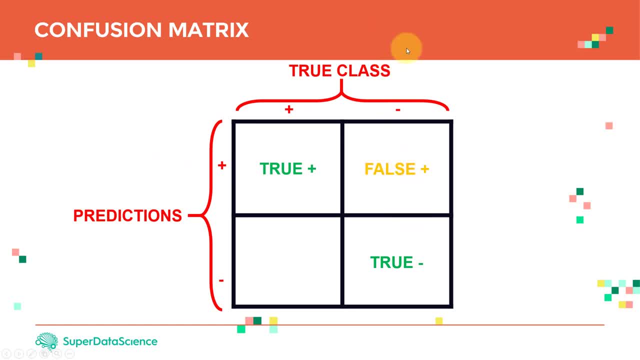 However, in fact, the patient was actually negative, which means the patient was actually safe to start with. He didn't have any cancer, okay, So that's why we call it false positives. The model messed up and he claimed that the patient has a disease. 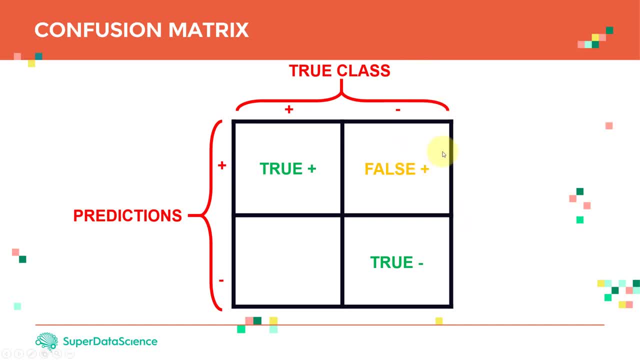 But in fact the patient was fine And this what we call a type one error. And now to the problem. now to the issue, which is what we call it false negatives, And that's why I highlighted it here into red, because that's a major problem in models. when it comes to models, 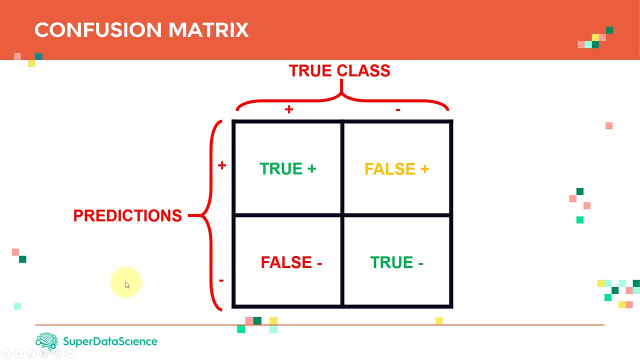 That's when the model predicted that the patient doesn't have cancer. So, you know, we collected data of the patient and we trained the model and the model said: you know what? This patient is fine. However, in reality, in fact, the true class was actually positive. 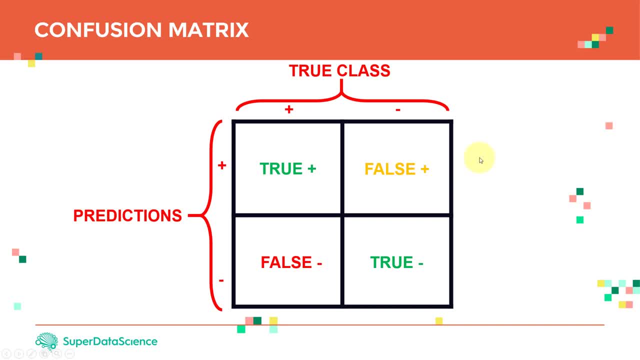 And that's a huge issue, because now the patient is in danger. He is not receiving any medication to stop the cancer or to stop the progression of cancer. So that's why we call this type one error and we call this type two error. 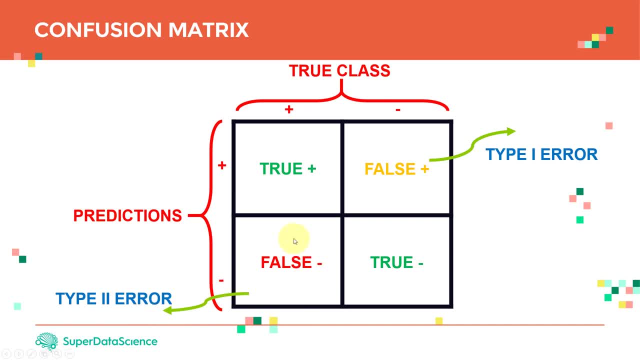 And it's a huge issue. type two error, And actually type two error as well, is huge. let's say, in any other application And let's say self-driving cars, for example, False negatives is a huge issue. Why? 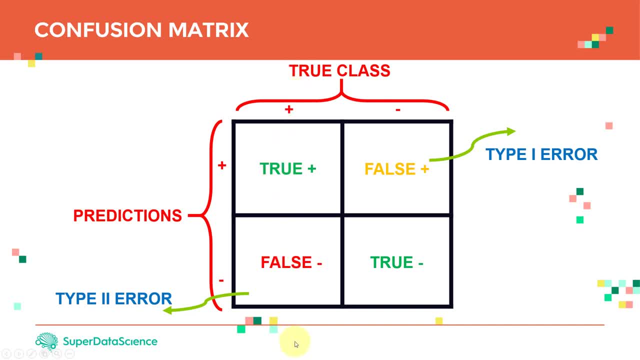 Because, for example, here we might, the true class might be positive, which means in fact, for example, there is a pedestrian. However, my network or my model said, you know what? There is no pedestrian. Okay, so that's a huge issue too. 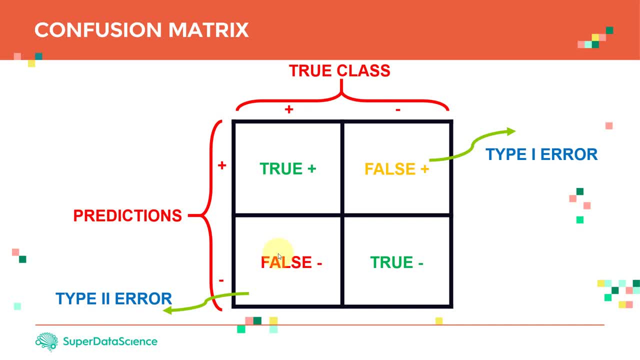 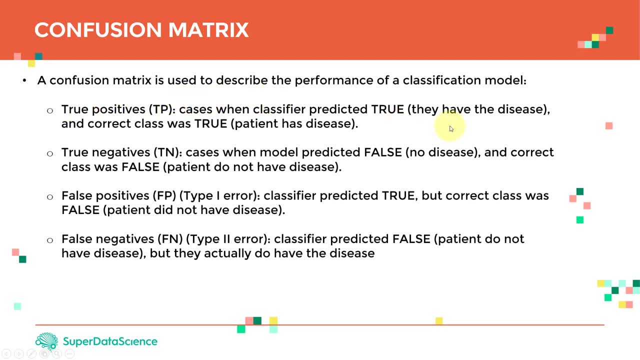 Again, you can apply the confusion matrix or these concepts in pretty much any classification application, All right. So a confusion matrix is used to describe a situation, It describes the performance of a classification model And we have true positives, true negatives, false positives and false negatives. 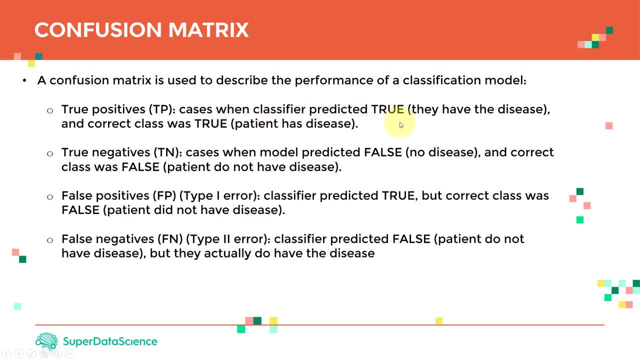 True positives are cases when the classifier predicted true, which means that they have a disease, and the correct class was actually true. In fact, the patient has a disease as well. True negatives is cases when the model predicted that it is false, which it has no disease, and the correct class was actually false as well. 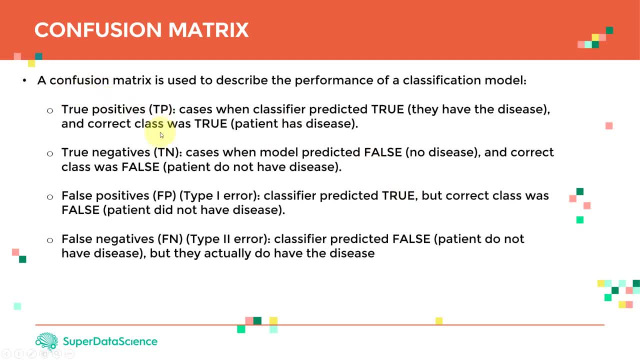 which means that the patient did not have a disease as well. So, true positives and true negatives, they are good. Okay, that's when the model actually get it right. Now to the problems. We have what we call false positives and false negatives. 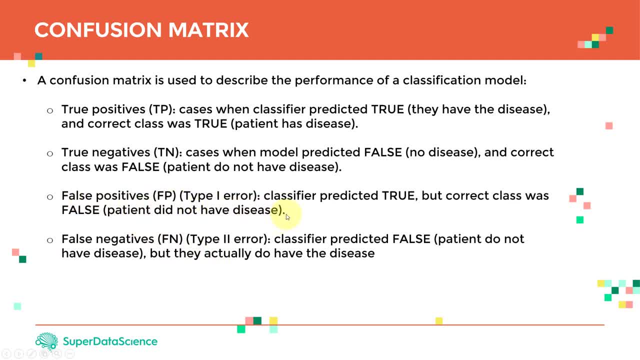 False positives are what we call a type one error. That's when the classifier predicted true, but the correct class was in fact false, which means that the patient did not have a disease to start with. Okay, Again, it's an error. 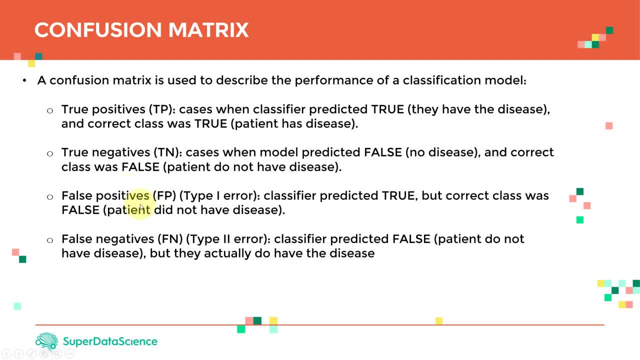 It's a mistake, but the patient is fine. That's what we care about. right, And that's why we call it type one error For false negatives. and that's type two error, that's when the classifier predicted false, which means the patient do not have a disease, but they actually do have a disease. 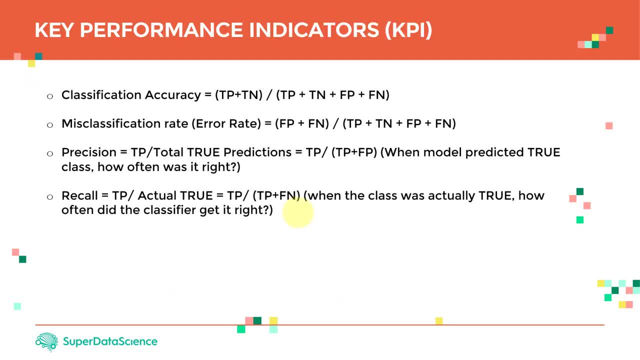 And that's the issue. That's a big problem, All right, So let's see how can we assess the performance of the model. So there's a lot of KPIs, or key performance indicator, when it comes to classification problems And when we apply the logistic regression classifier. 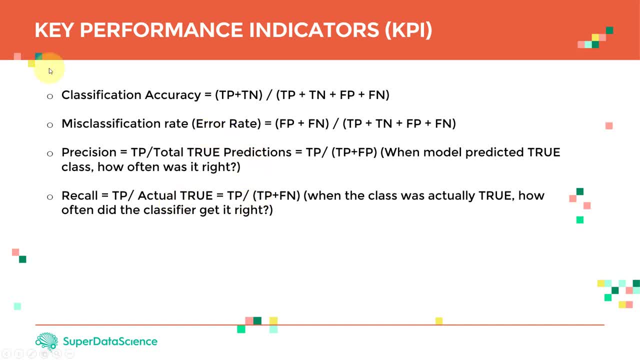 we are going to assess the performance of the model based on these. First we have our classification accuracy, which is true positives plus true negatives, divided by the overall number of samples. Simply put, we'll go back to the matrix. sum up these two. 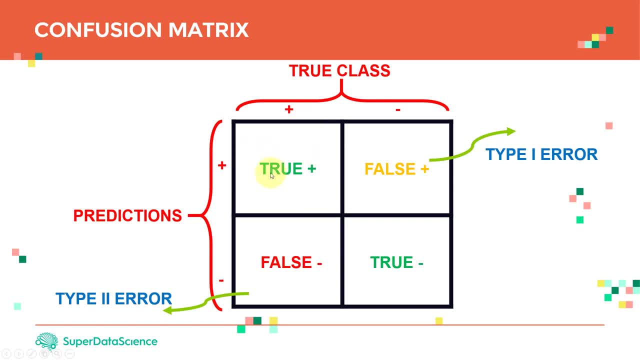 So we're going to sum up how many samples have been correctly classified as positive and as negative. So sum them up Divided by the overall number of samples, Divided by true positives plus false positives, plus false negatives, Plus true negatives as well. 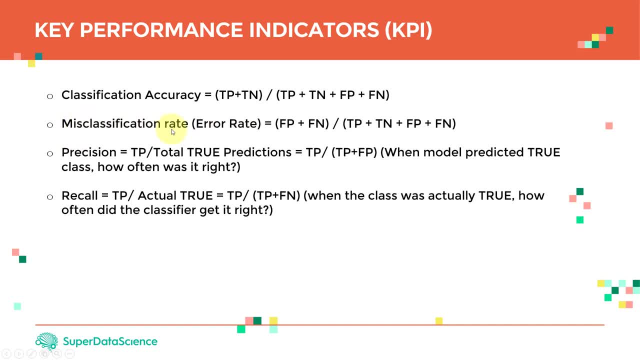 Okay, And then we have the error rate, or misclassification rate, which is false positives plus false negatives, divided by true positive plus true negative, plus false positive plus false negative. Again, we're going to count how many times we messed up, Okay. 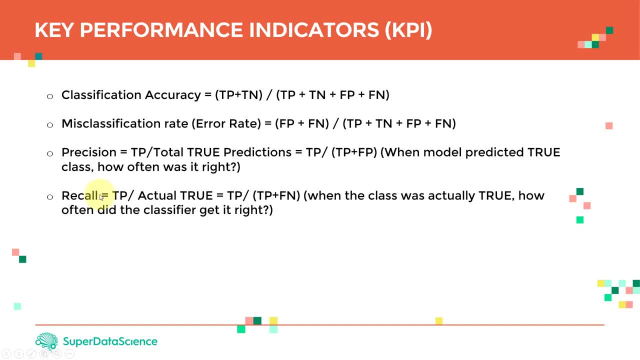 And then we have two important definitions, and we call them precision and recall. Precision is simply the true positives divided by the total true predictions, Which means it's simply the true positives divided by true positives plus false positives, That's when model predicted true class. 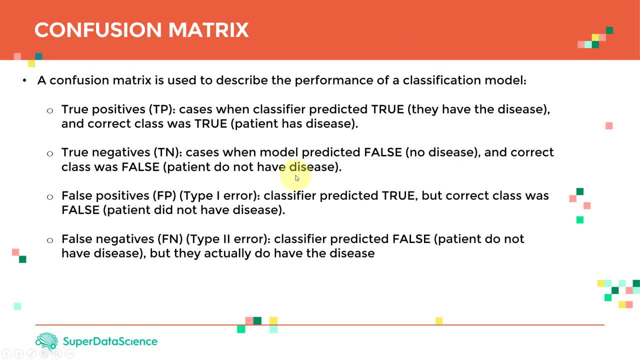 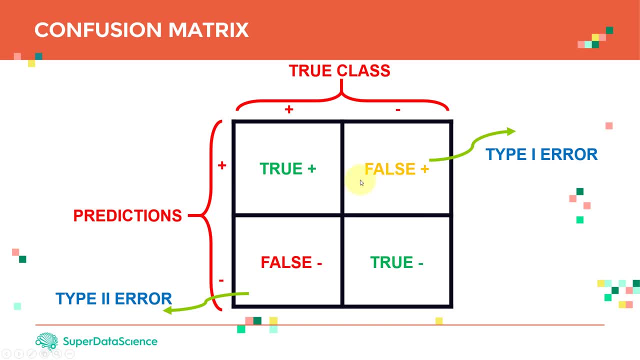 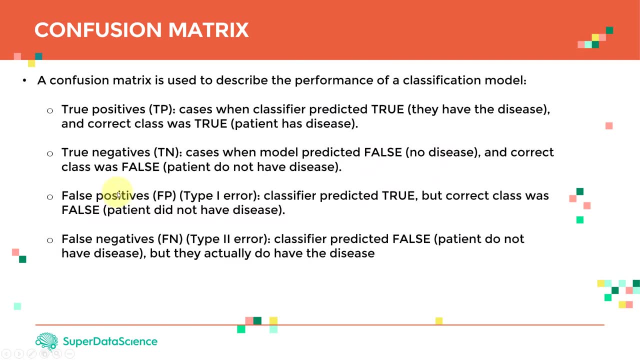 How often was it right? Okay, So simply, when the model said that I am positive here, how many times he was right? How much of the model was right, Which is simply true positives plus true positives plus false positives, And that's what we call it precision. 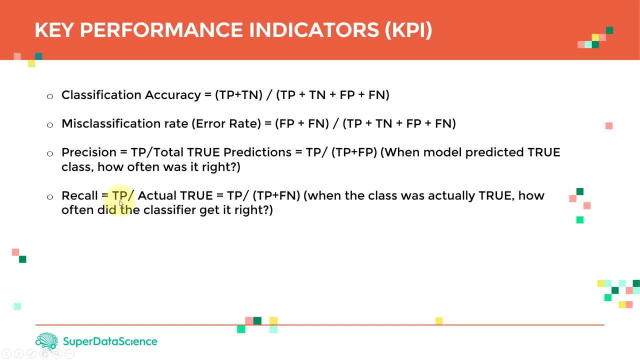 The next important definition is what we call recall, Which is true positive divided by the actual true, Which is true positive divided by true positive plus false negatives. And that's when the class was actually true. When the class was actually positive, How often did the classifier got it right? 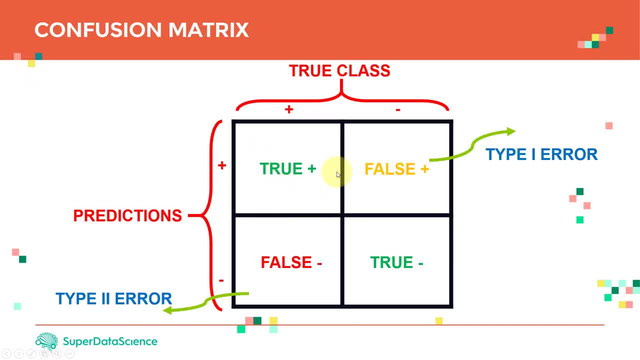 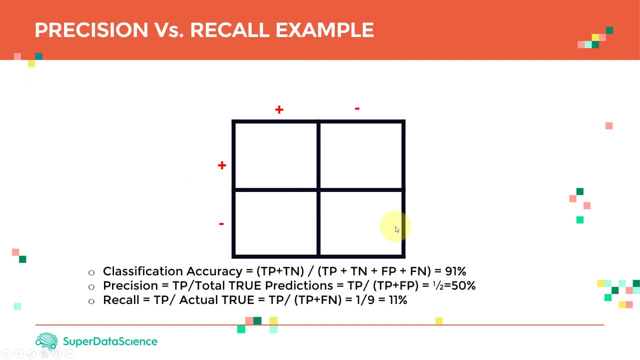 Okay, That's the overall idea. So we basically go here: divide true positives, divided by true positives, plus false negatives. Okay, All right, Okay, So let's take a look at actually practical example. I know it might sound a little bit confusing. 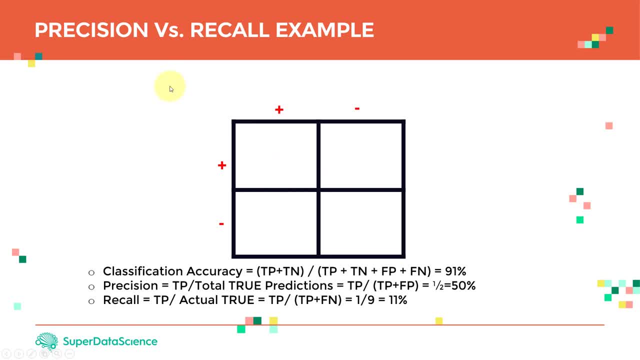 That's why I tried here to add an example for you guys to compare the precision and recall. Okay, Let's assume that I have a patient. Okay, And I have all these numbers in here. So let's assume that I have 100 patients. 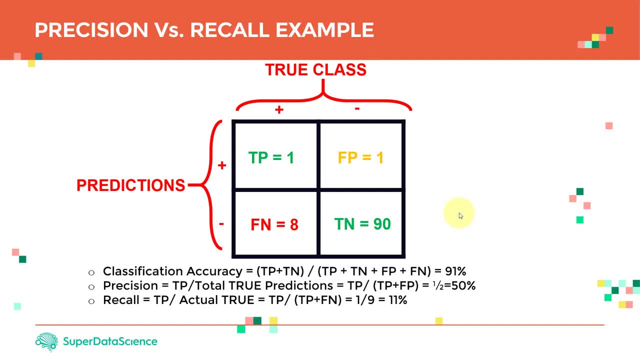 Okay, And in reality, okay, we have 91 patients that do not have cancer. Okay, And I have 91 patients who are totally fine, Everything is good. Okay, And I have nine patients that do have cancer. Okay, And the perfect model would be able to correctly detect these nine patients and isolate them. 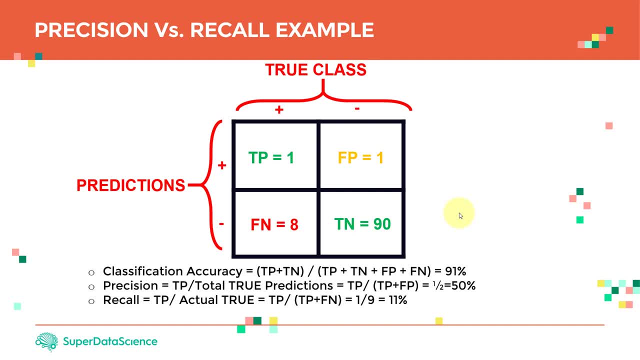 I'm going to say, okay, these nine patients have cancer and we need to treat them to basically clear the cancer and maybe, like, give them a chemotherapy or whatever medication to actually fix it up. Okay, All right, So let's assume that we have a model and that model gave me these results. 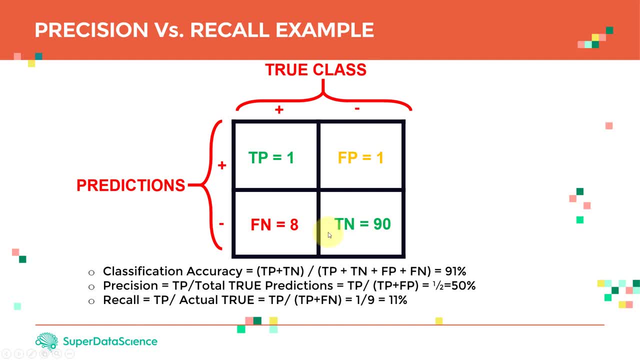 The model: true positives were equal one, true negatives were equal to 90,. false positives were equal to one and false negatives were equals to eight. So if you sum them up, you will come up with 100 samples, Right, Okay? 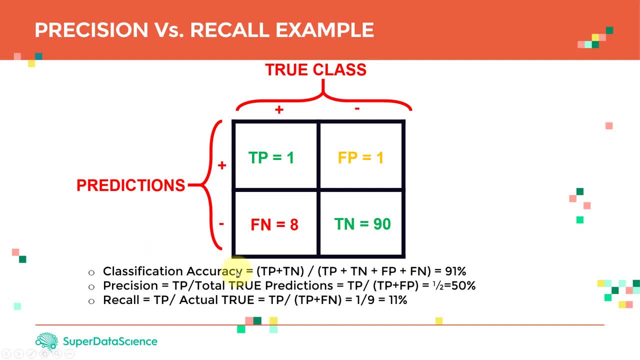 So first let's calculate the classification accuracy. So the classification accuracy: as I mentioned, we are going to count how many samples I was able to correctly classify. So I sum up 90 plus one, So true positives plus true negatives divided by a hundred, which is all samples summation. 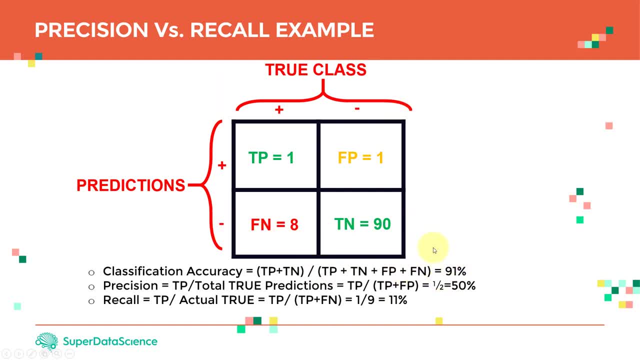 of everything, We'll come up with 91%. So if you take a look at it you would say, wow, that's amazing. You know. that means you know like the model is 91% accurate, Everything looks good. 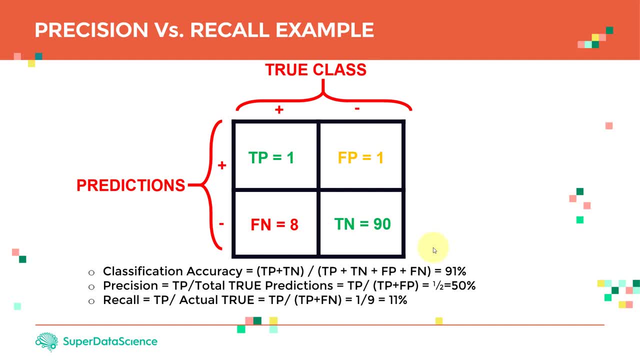 The model has able to correctly classify 91 samples out of a hundred. However, if you dig a little bit deeper, this model is accurate. It's actually garbage. Okay, You cannot use this model in practice, Why? And that's where precision and recall comes into play and they can expose the limitation. 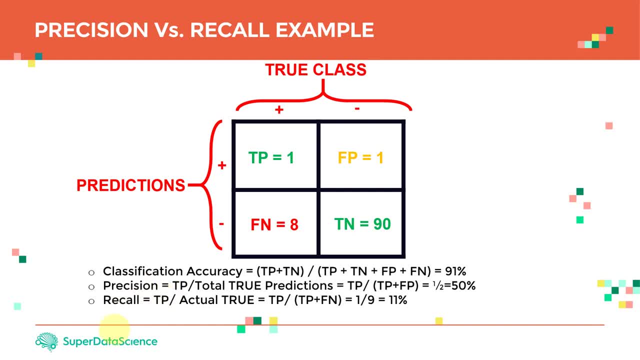 and shortcomings of the models. So precision: is true positive divided by total true predictions. So is simply one which is true positive divided by true positive plus false positive. So I'm going to divide one divided by one plus false positive, One plus one, which means it's half or equal 50%, which means that basically, the model 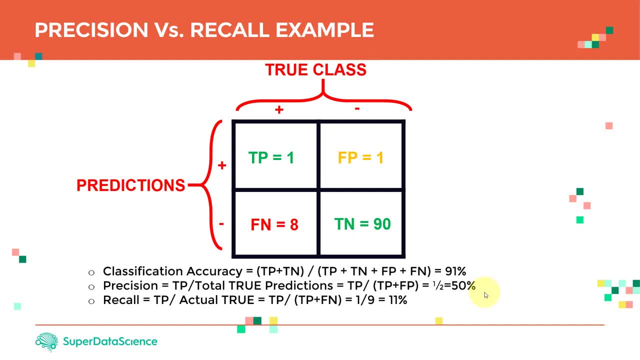 is 50% correct, which is horrible. This results are really terrible, which means that, again, when I say precision, that means when the model said that it's positive, when the model said that the class was positive here in the row, how many times it was actually right? 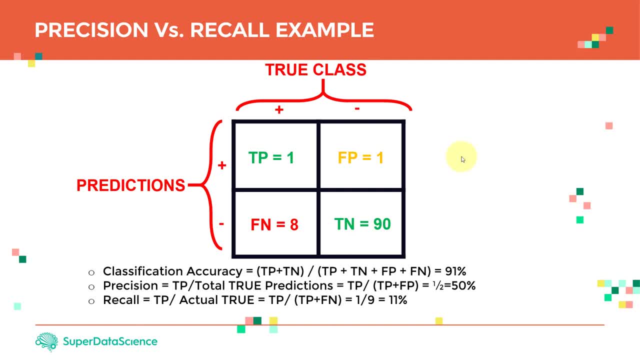 You will find that. you know, the model said that there were only two positive cases and basically the changes, The differences of, like it's, the precision was only 50%, So it only got it 50% right, which is terrible. And now to the another important element as well, or important metric, which we'll call. 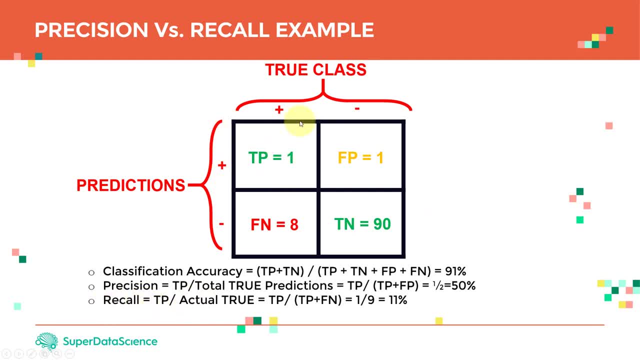 a recall Recall is simply our true positive, Okay, Divided by the actual true samples, which here we have two positive divided by a true positive plus false negative, which is one divided by nine, which is one plus eight. So here we have 11% recall, which is that mean that this model is actually again the 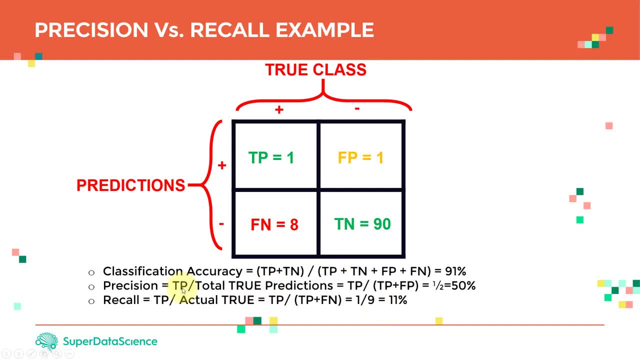 performance is really bad And, as you guys can see here, recall, simply try to obtain, when, basically the how many samples, how many of the nine samples that we have, how many of these cancer patients I have been able to correctly classify. So here I have been able to correctly classify only one sample out of nine samples, which